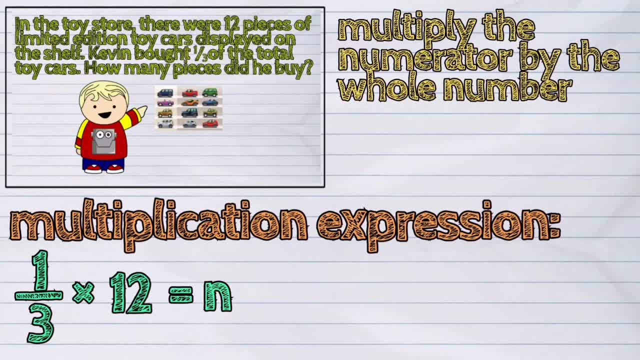 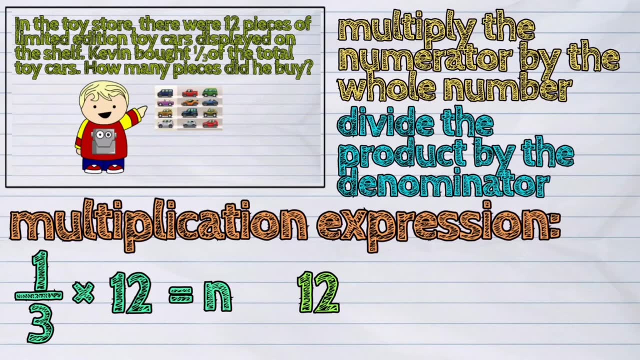 So it's one times twelve. This is equal to twelve. Next, divide the product by the denominator. Our product is twelve And our denominator is three, So it's twelve divided by three. This is equal to four. 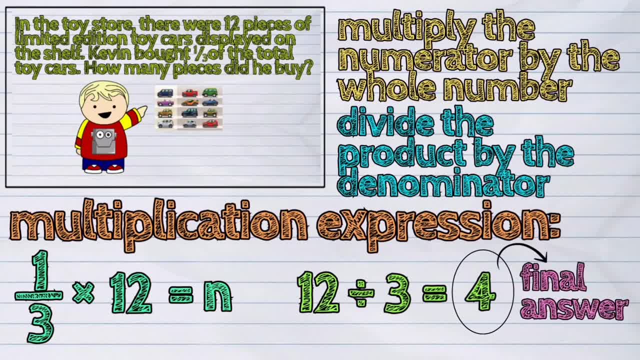 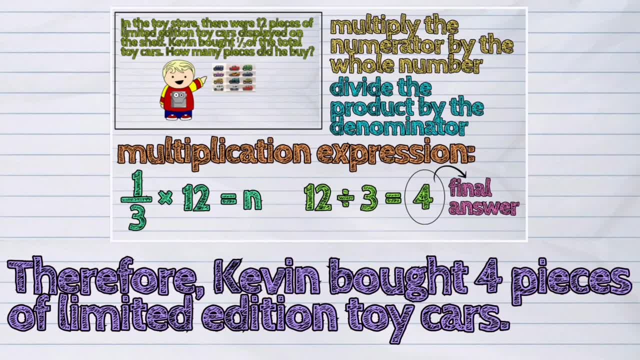 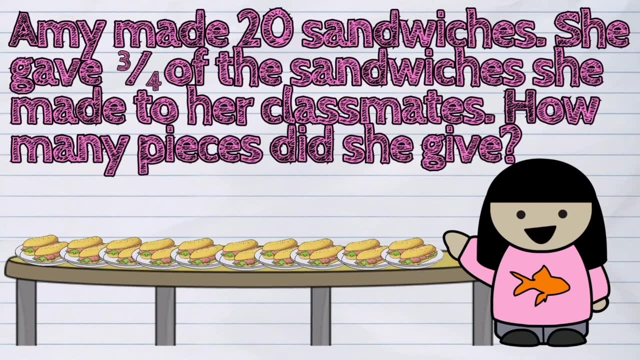 Four is our final answer. Therefore, Kevin bought four pieces of limited edition toy cars. Another example: Emmy made twenty sandwiches. She gave three-fourths of the sandwiches she made to her classmates. How many pieces did she give? How many pieces did she give? 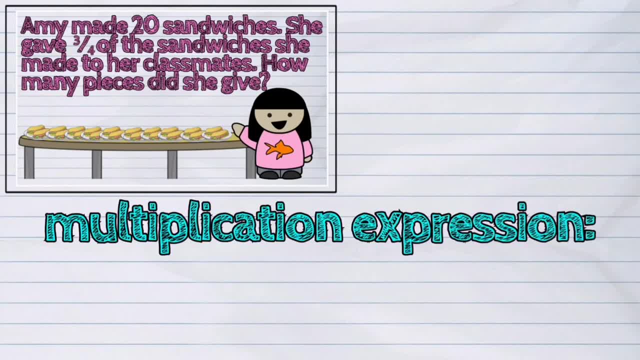 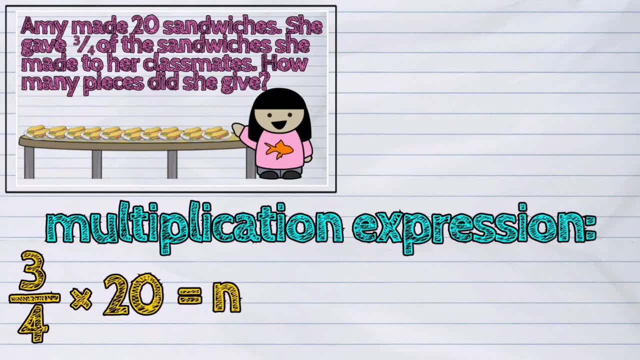 Again. let's write the multiplication expression, which is three-fourths times twenty. We can also put a denominator one under the number twenty for an easier solution. So it's three-fourths times twenty over one. Three times twenty is sixty. 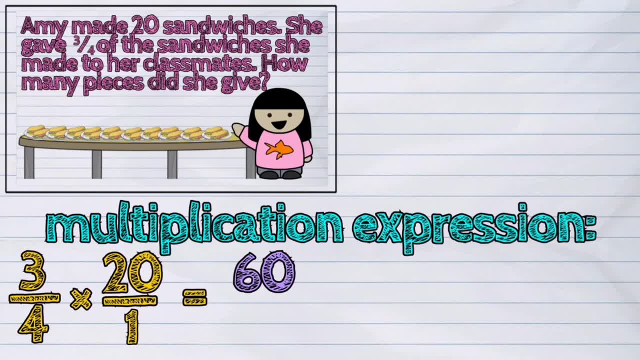 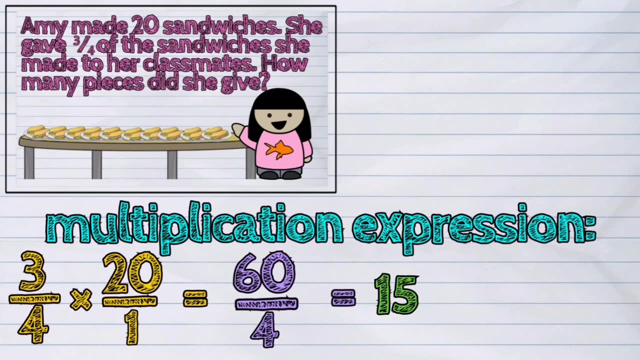 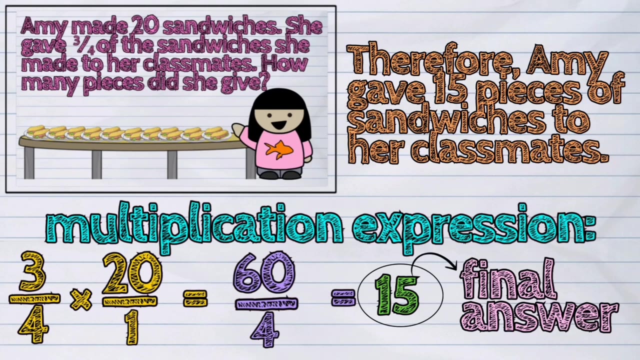 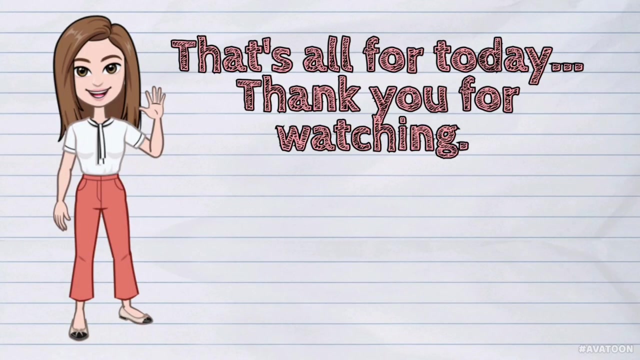 Four times one is four. Next is: divide sixty by four. The answer is fifteen. Therefore, Emmy gave fifteen pieces of sandwiches to her classmates. That's all for today. Thank you for watching. Please don't forget to like and subscribe. Till next time.